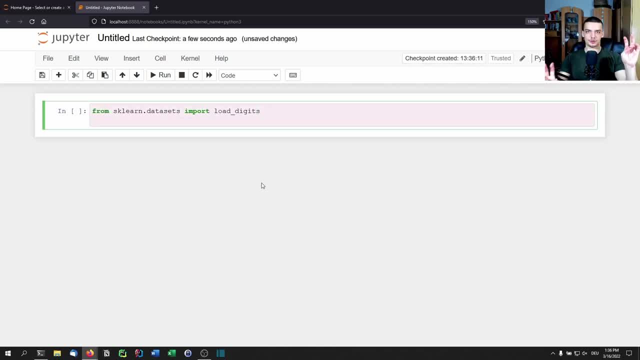 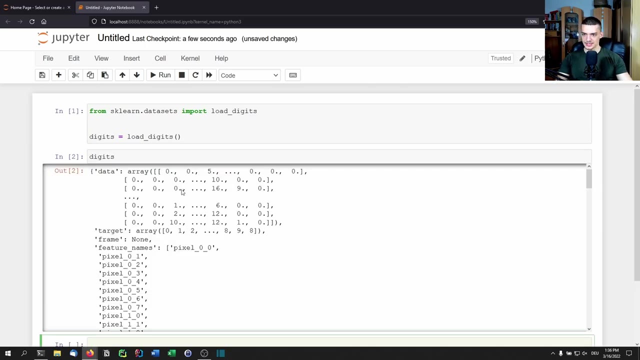 load the MNIST data set, which is like the Hello World data set for machine learning. So we can say digits equals load digits And essentially those are just handwritten digits. Let's just see what they look like. So we have data, we have target. maybe we should look at the 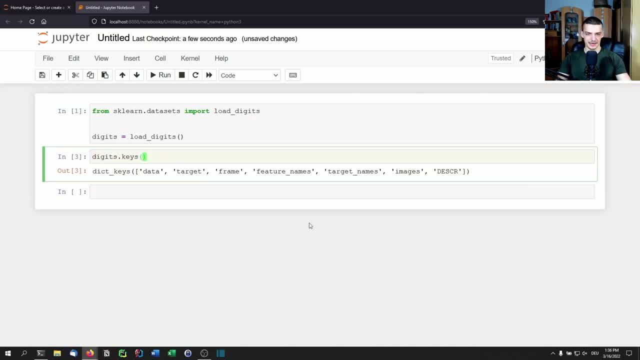 keys. First, we have data target frame and a couple of other things. We're interested in the data, those are the pixels and the target is then the label, So the respective digit that is displayed. So we can actually go ahead now and visualize this by saying: for data. 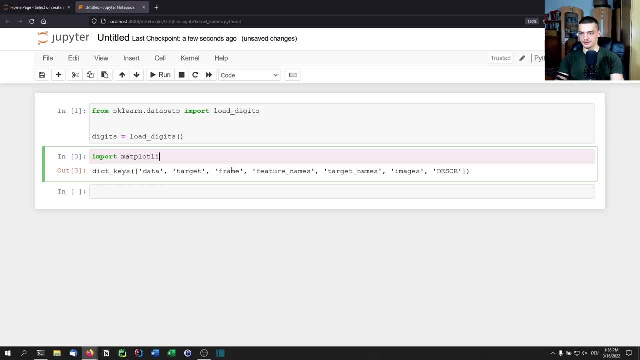 I'm going to need an import. import matplotlibpyplot, SPLT. By the way, all these libraries, you should have them. you can install them by using pip. So pip install matplotlib, pip install sklearn, pip install numpy, pip install pandas and so on. if you don't have, 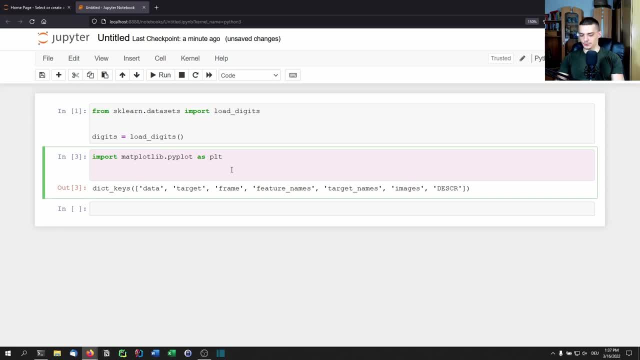 them in the command line, And what we're going to do now is we're going to say plt- imshow, And we're going to show the pixels of digits, dot, data, zero. So the first one, and we're going to have to reshape this Now. the format here is not the classic 28 by 28.. I think it is 28 by 28.. 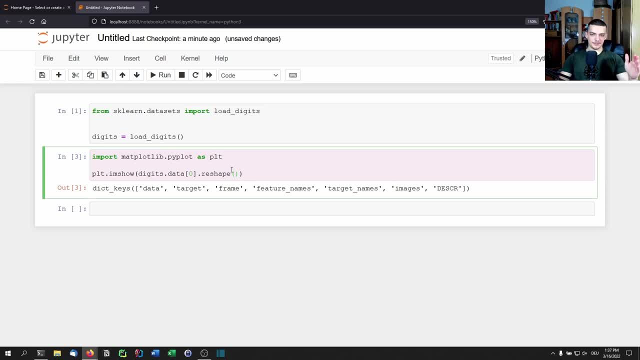 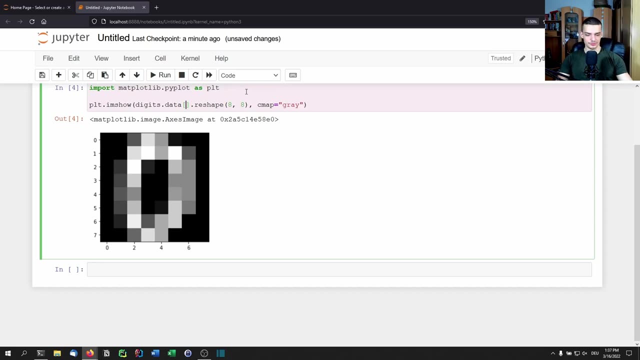 In this case it's eight by eight, So we have eight pixels times eight pixels, 64 pixels in total. So we're going to reshape this like that And we're going to say: the color map is going to be great And this is a zero, for example. we can also go to something else, like 20, for example. 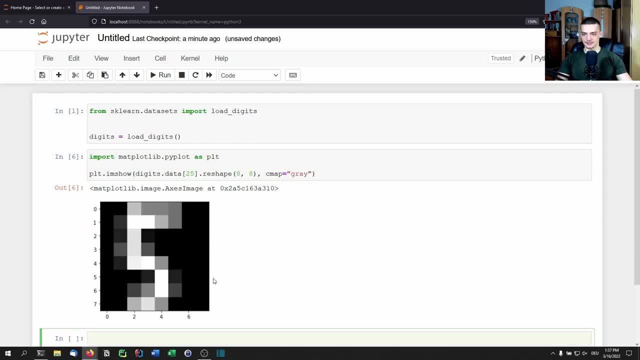 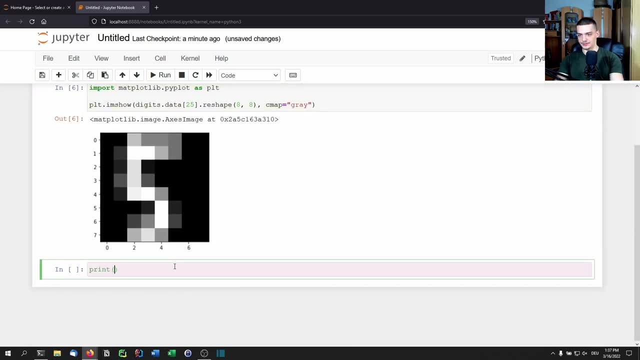 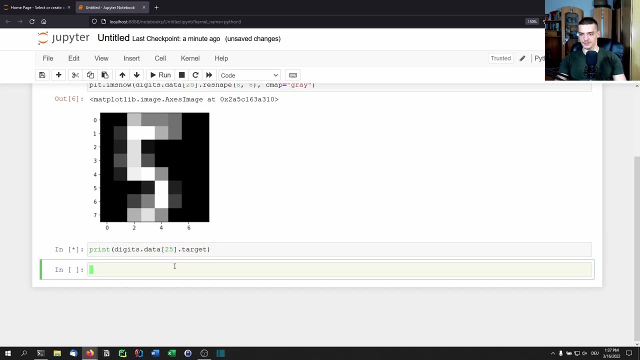 and this is also zero, then 25.. This is going to be a five. So we have these digits here And we also can see that if I go and print now digits: data 25 dot target. Oh sorry, this was wrong. Data targets 25.. This is what I'm looking. 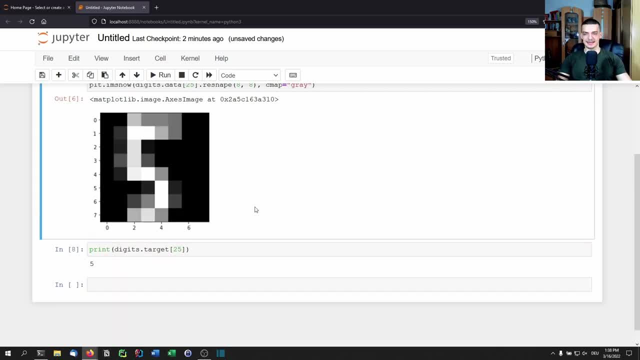 for This is going to be a five. So this is the label, those are the pixels And this is a simple classification task, right? So you choose a model and you train them all on one part of the data, to test it, to evaluate it. on another part of the data, how well it does a predictions, and with 64 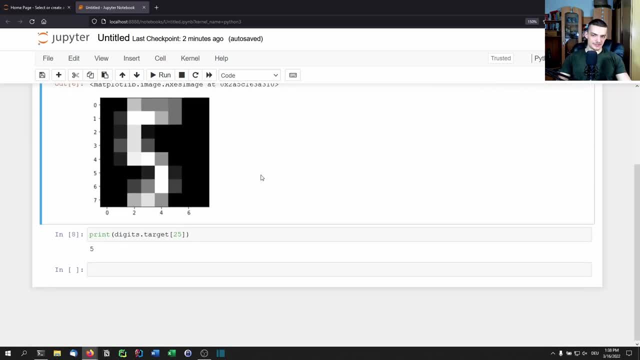 pixels. this should be quite easy. So this is not the topic of today's video. how to do that? I have, I think, two videos on that, And this is like a hello world example for machine learning. This is just the example that we're going to use to explain precision and recall, So let us just 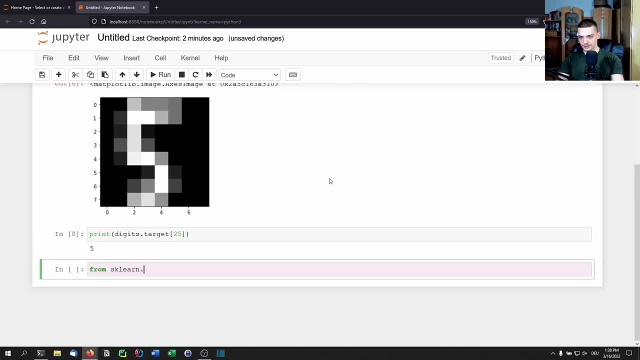 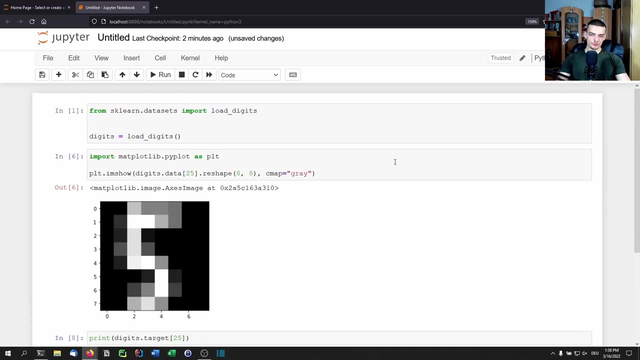 build a simple model to predict that we're going to say, from SQL learn dot model selection, We're going to import the train test splits and from SQL learn dot neighbors, we're going to import K neighbors classifier And we're going to do not a general digit classifier Because, in order to explain, 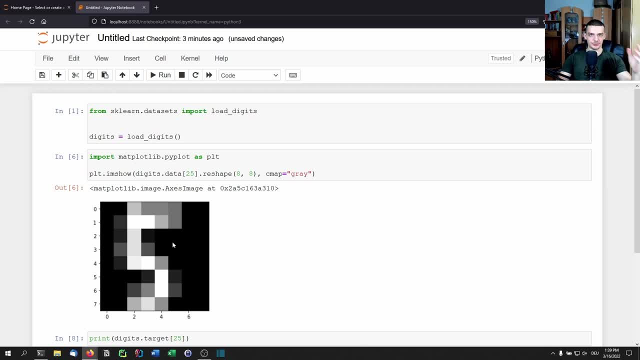 precision and recall. we're going to use here a binary classifier, So either yes or no. And of course when we have 10 digits, a yes and no classifier doesn't work on all the digits. So we're going to pick one digit And then we're going to use a binary classifier And then we're. 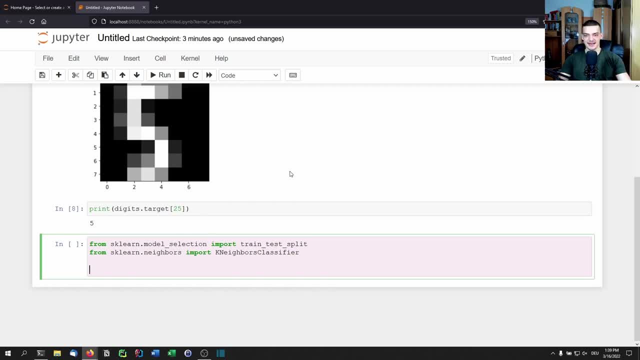 going to create, for example, the eight. we want to classify if something is an eight or not. So essentially we can say: eight underscore CLF. for eight classifier is a K neighbors classifier And the x, the x values are going to be just digits, not data. So the pixels and the y data is going. 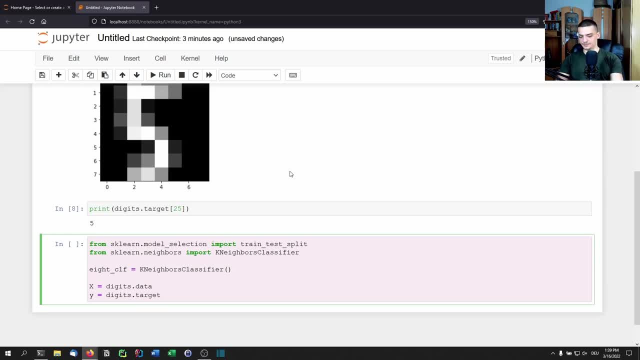 to be digits, dot targets being equal to five as as a condition. So this is going to return zeros and ones. Actually, not five, sorry. eight is going to return zeros and ones. So whenever a digit is an eight is going to return. 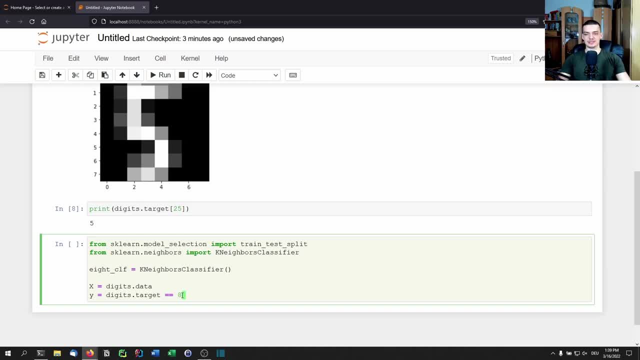 a one, And if it's not an eight, it's going to return to zero. So we make it a binary classifier instead of a digit classifier. So it's not going to tell us that this is a five or a four or six. 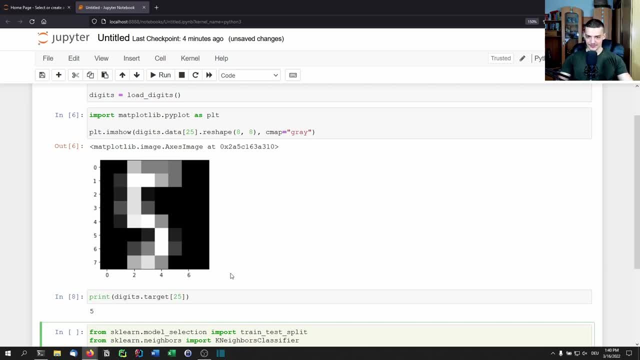 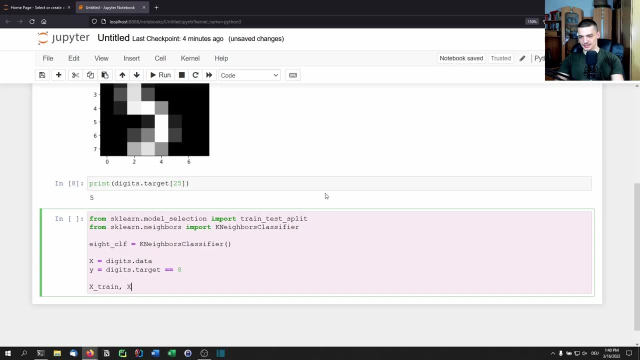 it's just going to say yes or no. Is this an eight or not? Again, this is just the example that we use to explain precision and recall. Now we're going to split that data into x train, x test, y train, Y test by calling the train test, split x, y And let's pick a test size. Now this is going to be. 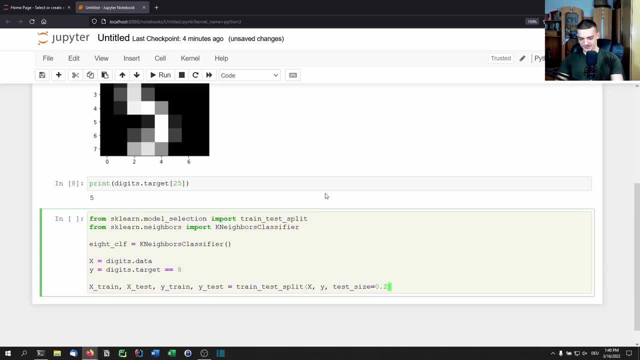 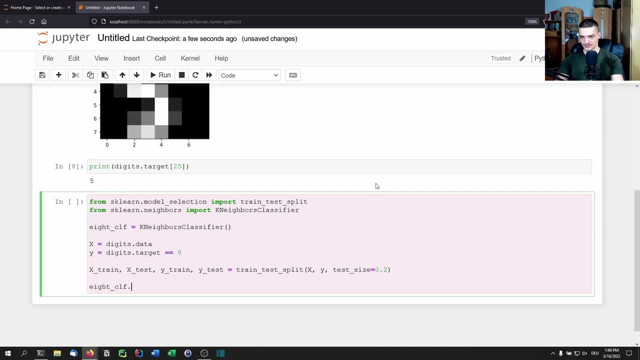 quite simple. So I think we're going to get close to 100% accuracy, But we're going to go with 20% test size to start with And then we're going to just train a classifier. So a CLF dot fit on x. 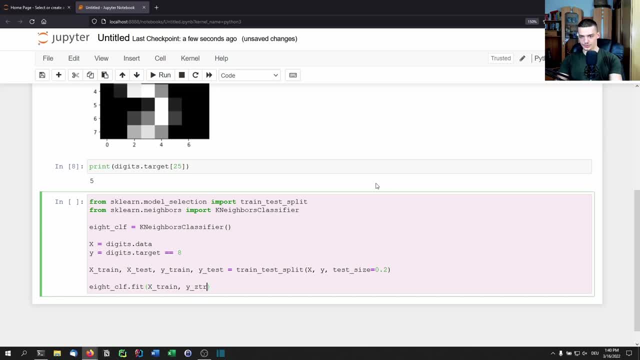 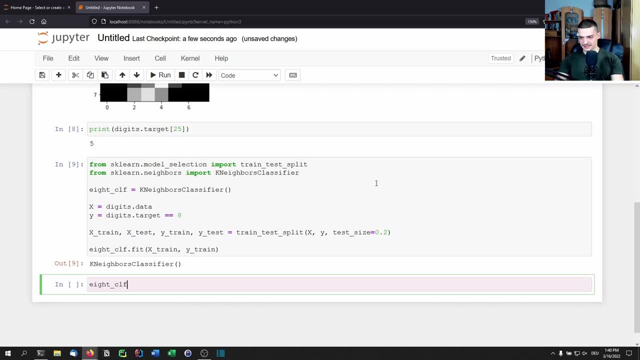 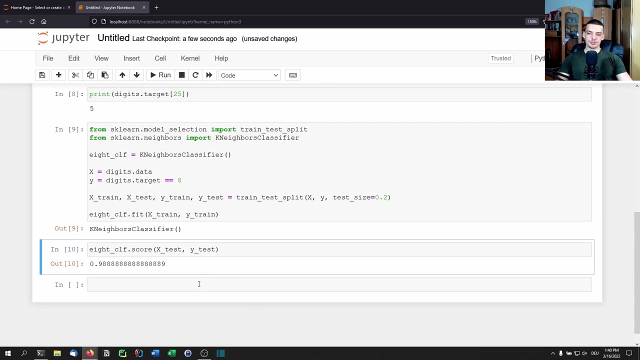 train and on y train. Now what is important here is that when we now say, for example, let's evaluate this classifier eight, eight, CLF dot score, x test, y test, this is going to give us a score, in this case 98.888%, So pretty high score. But what you need to understand about the score is that this is 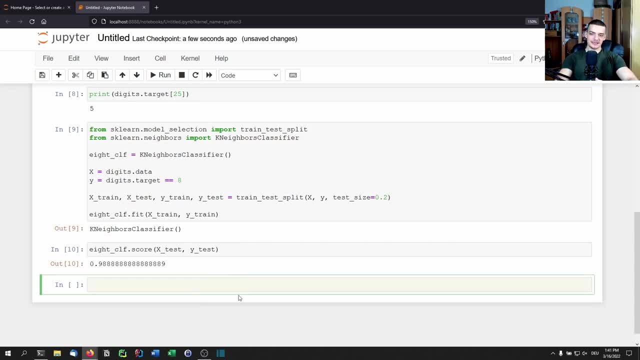 accuracy. So accuracy is defined as: how many samples did I look at and how many of them of them that I get correctly, So we can calculate the score ourselves by just by just saying: Okay, give me the predictions. So manually, we're going to say why predictions is the eight classifier, dot predict. So 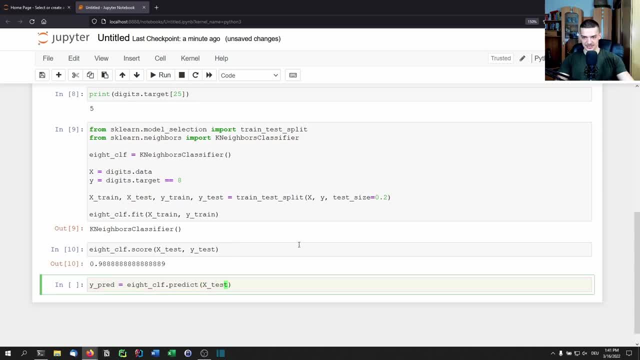 based on the training data. here we predict now the test data, which is the same as scoring, but we're going to do the comparison manually to understand what is happening And we can now say correct basically means that we get the sum of the correct classification, of the of the correct. 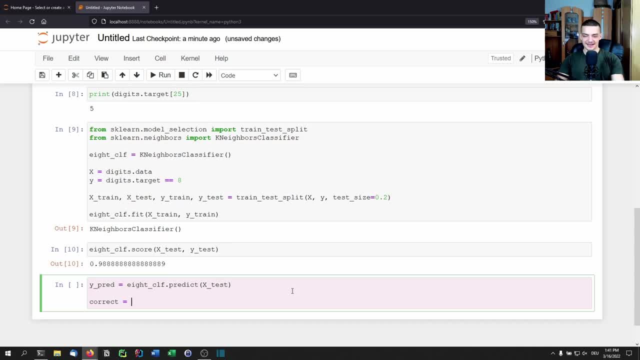 classifications. Oh sorry, this is one step ahead. What we want to get, what we want to do to get the correct classifications, want to compare the y predictions to the actual y test data. So this again is going to give us zeros and ones, or one every time when those two are the same, and a zero. 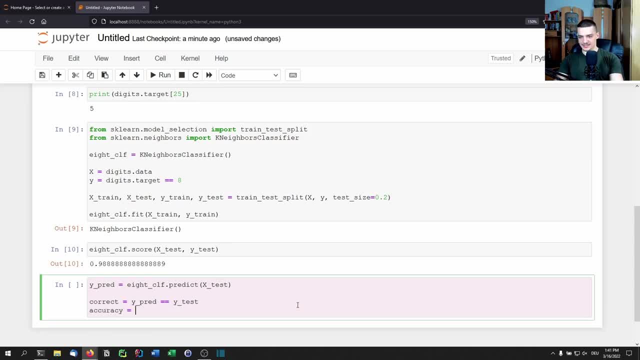 every time they're not. so we can get the accuracy by saying sum of correct. So sum all the ones divided by the length of correct by basically everything. So this gives us the percentage, and now I can just go ahead and print the accuracy. There you go. 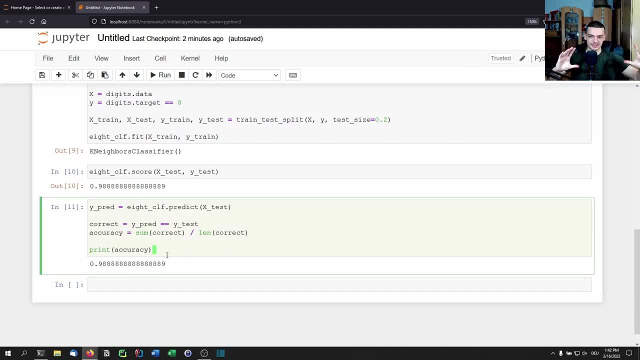 So this takes all the samples, all the instances, how many of those it will get correctly as a percentage. This is the accuracy, And accuracy is actually quite a good metric to look at. However, sometimes it's going to be not enough And sometimes it's going to be misleading, And oftentimes we also want to have more detailed. 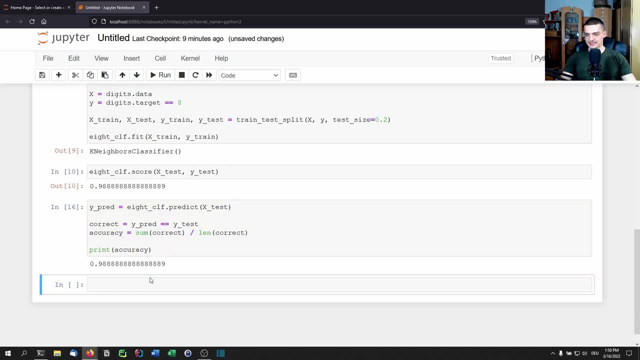 information about the models performance. Let me show you a simple example here. Let's go ahead and say: now the y values, the y predictions are not going to be based now on the eight classifier that we trained. we're just always going to say that whatever we see, it's not an eight. so we're going to produce a prediction set of only zeros. we're going 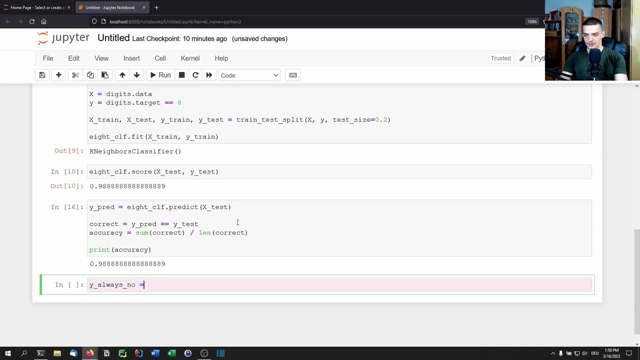 to say y always underscore. no is going to be zero. So basically no for length of x tests. So for each sample that we see while testing, we're going to say this is not an eight, this is not an eight, this is not an eight, and so on, And then we can. 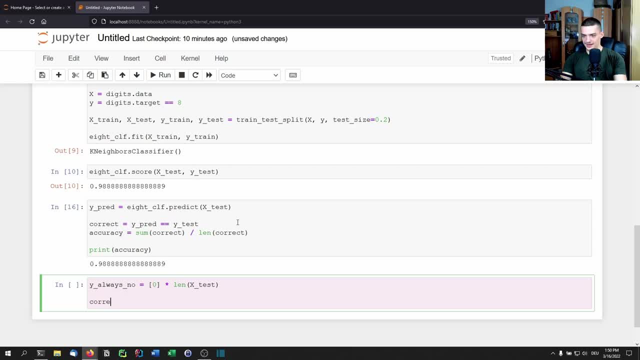 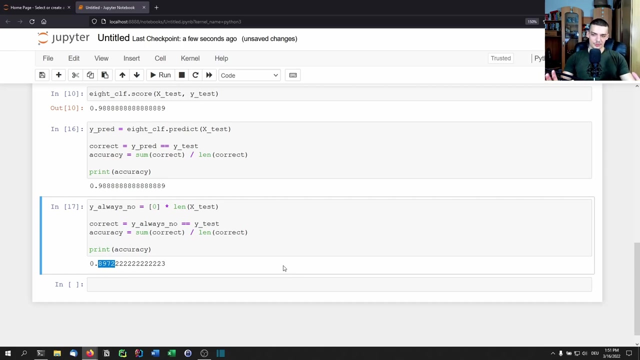 go ahead and basically say: the correct classification are going to be y, always know being equal to y test, And the accuracy is going to be the sum of the correct classifications, using that strategy, divided by the length of the predictions, And then we can just print the accuracy And what you see here is that we get 89.72% accuracy, 89.72% of the. 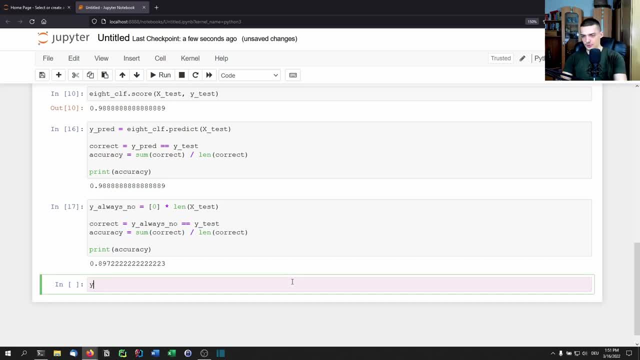 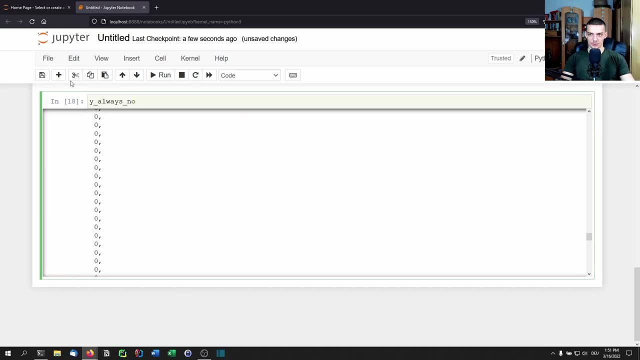 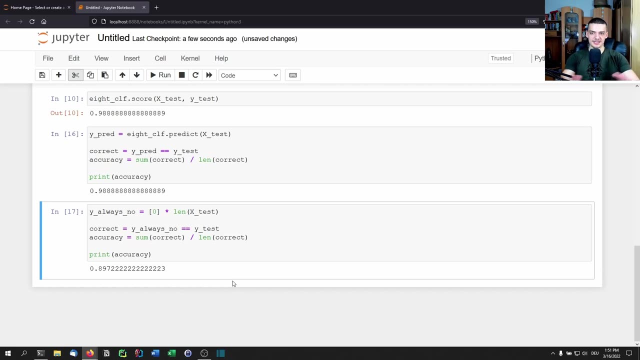 time we do the correct classification, even though our prediction set looks like that only zeros. always saying no, no matter what we see, which means that whenever we see an eight, our classification is wrong. We basically always, whenever we see eight, we say no, no, no. But 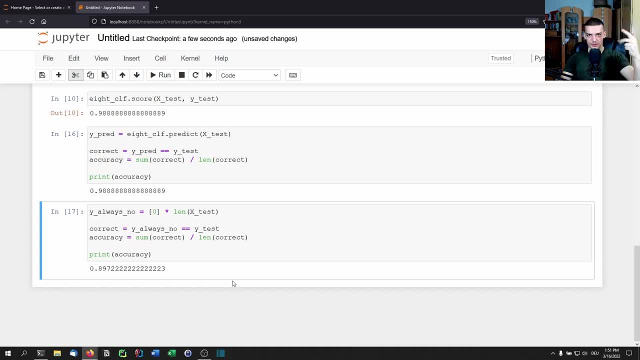 every time it's not an eight, and this is way more common with 012345679.. All these cases we make the correct classification. So we have a stupid classifier, but it works. it has a high accuracy. However, this is not a good model, then, because 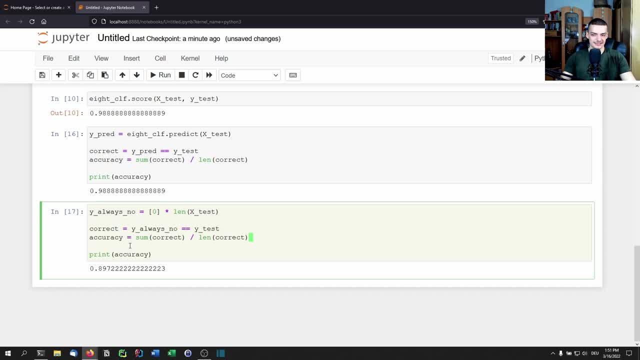 every time we see an eight, we don't recognize it. it doesn't recognize eights at all, it doesn't have any intelligent, And because of that we can use precision and recall to actually determine more specific metrics, because the recall, for example, is a metric that tells you okay from. 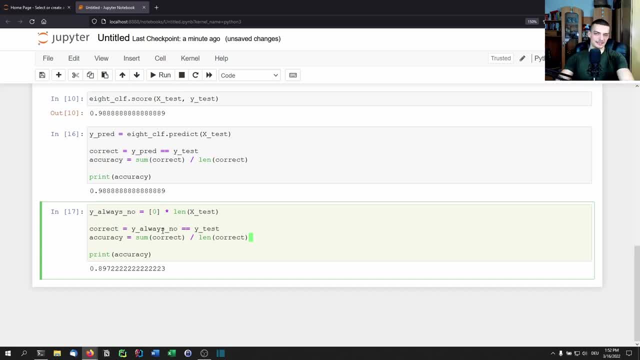 the. whenever you see a correct sample, in this case an eight, an actual hit, how many times or how much, how much percent of the times you see an eight, do you actually recognize it as an eight? this is the recall. in this case, it would be 0%, Because we see a couple of eights in zero times. 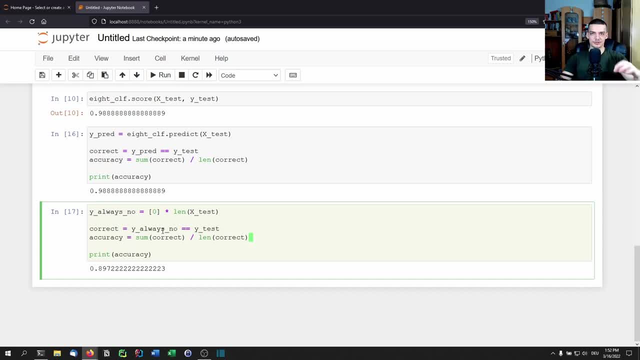 we say, yes, I recognize an eight. the recall is zero. the recall is very bad, very low Precision, on the other hand, says: when you say something is an eight, how many times are you actually right? So how many times when you say something is an eight, Is this actually an eight? 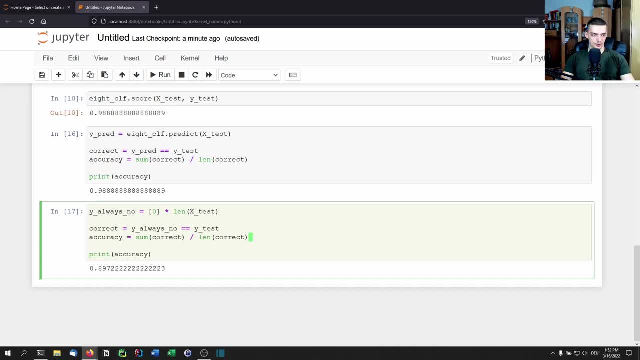 And we're gonna do that here first of all by just importing, or actually let's do it from scratch first, And for that we're going to need a confusion matrix. So the confusion matrix essentially is telling you your misclassification. So we're going to say from sklearnmetrics. 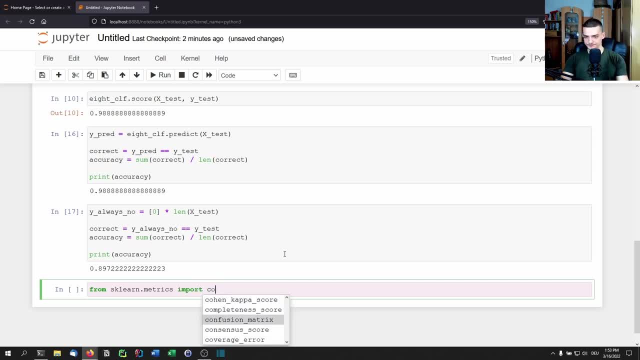 we're going to import the confusion matrix And then we're going to say confusion, Confusion equals confusion, Confusion matrix of. and we're going to use the k neighbors results here. So x, what was it? y pret and y test, And now we can print that And you can see what this looks like. 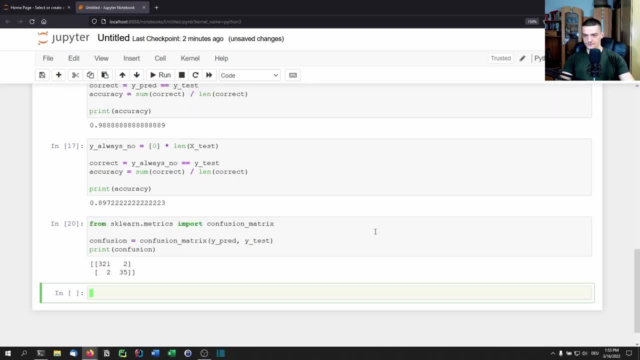 Confusion matrix. no, actually not the confusion matrix, the confusion. there you go, And in this case let me just look this up here, because I always forget how this is structured. Now the right column. so two and 35,. 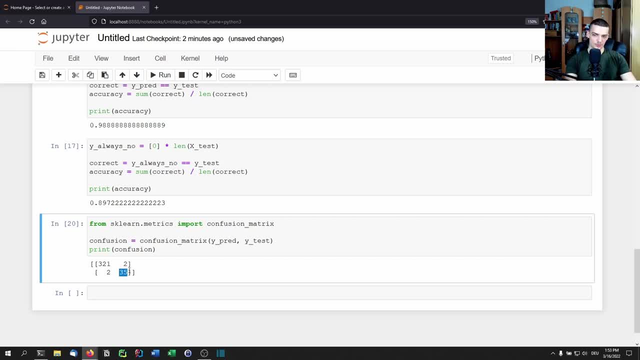 means we predicted. yes, So right is when we say something is an eight. Left is when we say it's not an eight And the top row means that it is not an eight And the bottom row means it is an eight. So basically, this means that here we have the correct classifications where we said: 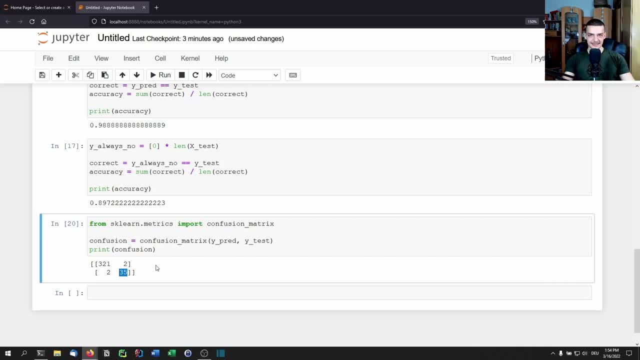 35 times we said that it is an eight and it was actually an eight. Two times we said it is an eight but it wasn't an eight. Two times we said it is not an eight but it was an eight, And 321 times we said it's not an eight. 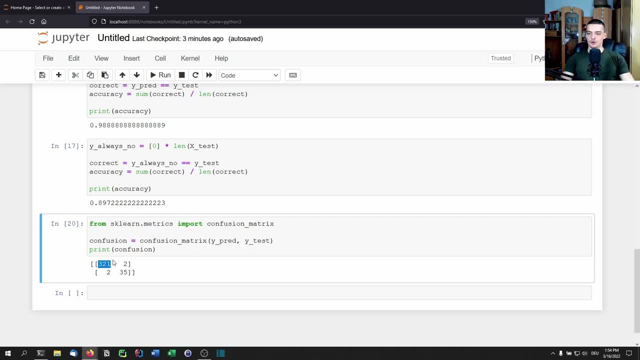 but it wasn't, And it also wasn't an eight. So those two numbers here are correct And those are the misclassifications- either true, false positives or false negatives. And based on those things now we can actually go ahead and compute precision and recall. So, as I said, the precision. 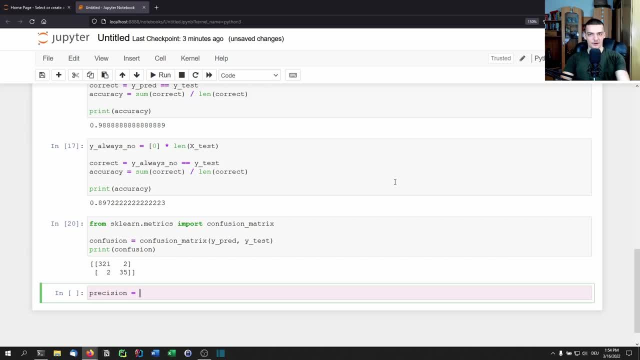 is essentially: when we say something is an eight, how often is it actually an eight? And because of that we're going to pick this value here. So those are the correct true classification. So when we say it's an eight and it is also an 835 times, 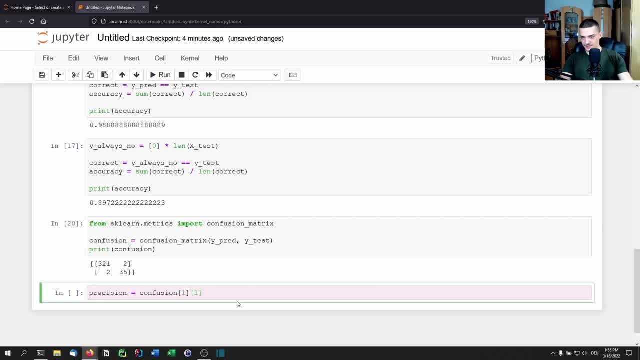 so confusion: one one, because we go into the second and second, one one confusion. and then divided by so the amount of true positives, divided by the amount of true positives and false positives, So confusion: one one and the false positives are zero one here. 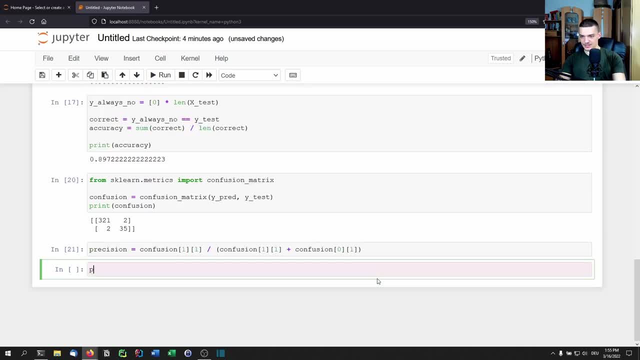 There you go, And this is now the precision. So we can go ahead and say the precision in this case 94.59%, which means that when we say something is an eight, 94.59% of the time we are right. 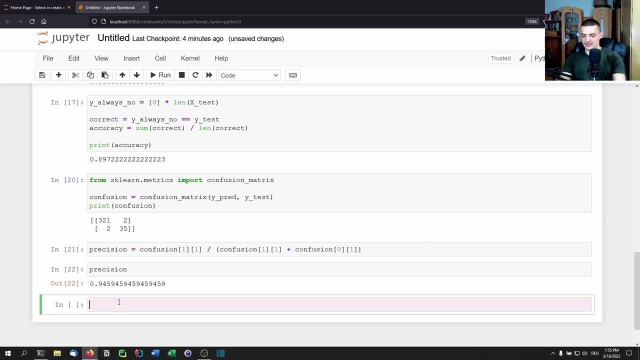 This is the precision There we go. recall is now what we also said: when something is actually an eight. so when we see an actual eight in front of us, when the model sees an actual uh eight in front of it, how often does it actually recognize it? so how often does it not miss an eight? you could also say: and for that we 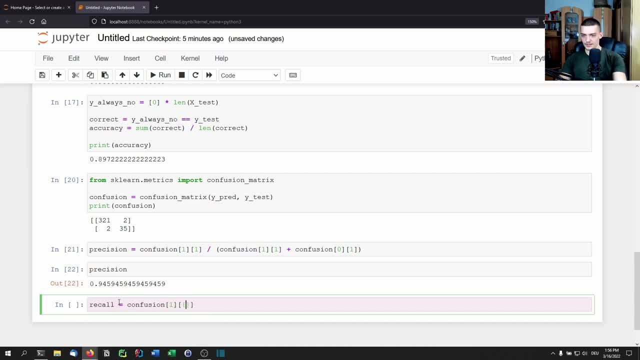 take again the true positives. so how often it recognized the correct eight divided by also again, how often it recognized it correctly and how often it was shown without to be recognized. so one zero, which is this here. and i think in this model, here the precision and recall are the same. 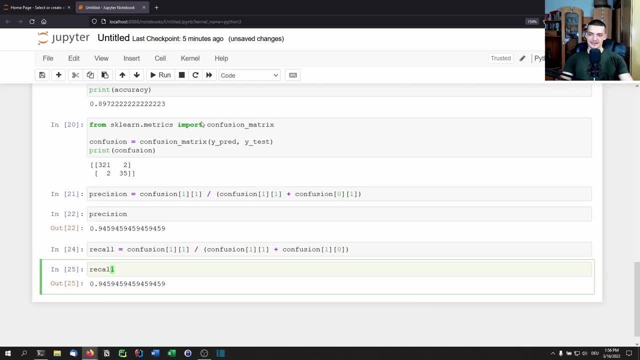 because we have two and two, there you go. but it doesn't have to be like that. this is just in this case, because here we have a two and here we have a two, and we take this plus this, and this plus this, and this is the same result. but it doesn't have to be like that. it doesn't have to be like: 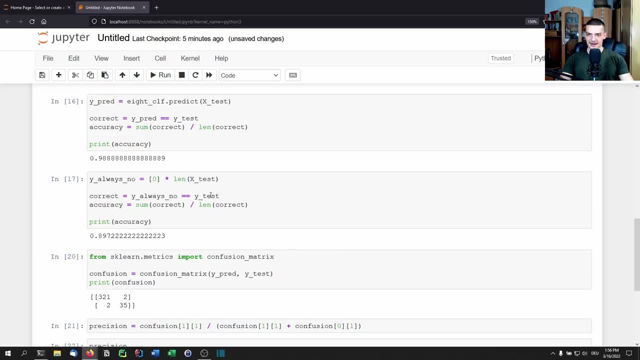 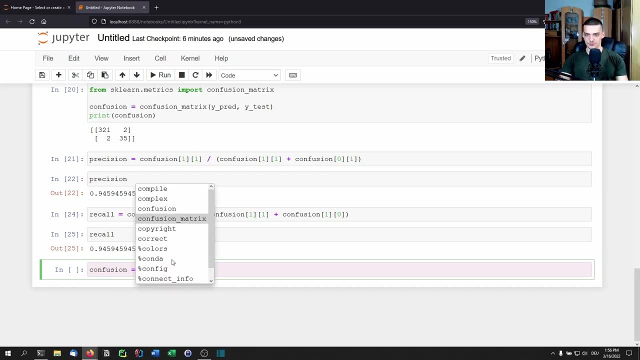 the case- and let me show you how this looks here- when we have the always no predictions that we talked about. so i can say here confusion equals confusion matrix, and we're going to say here now why always no and why test? so our primitive strategy and the confusion matrix looks like that. 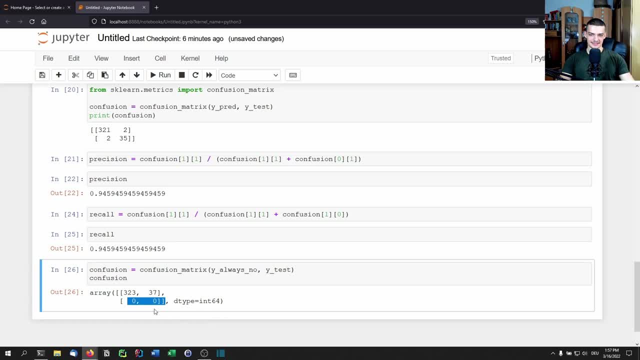 we never say that this is an eight. so the whole bottom um, so the whole bottom list, here is everything. because we never say yes, And because of that we can never make the mistake of saying yes while it's not true, But we also never say yes when it is true, And because of that, 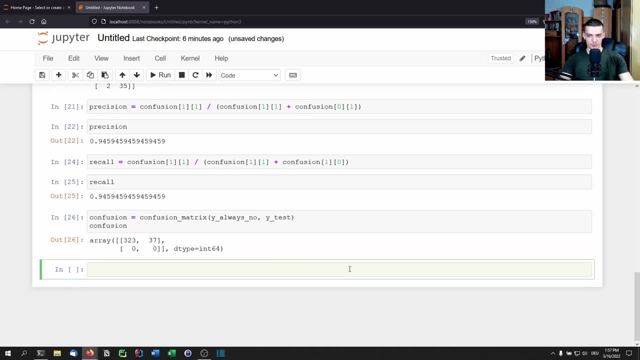 if I now go ahead and for this we're now not going to do it like that- we're going to import the respective SK learn modules. we're going to say, from SK learn dot metrics, we're going to import the precision score and a recall score, like that, And we're now going to say precision. 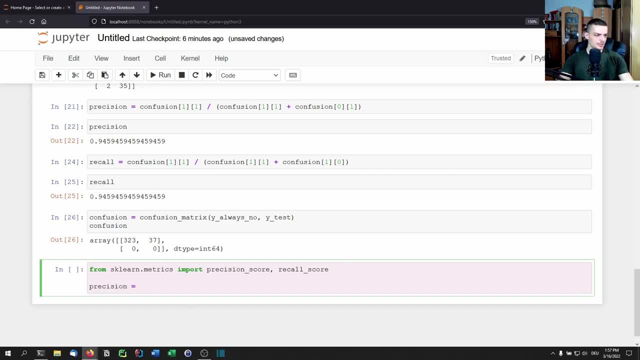 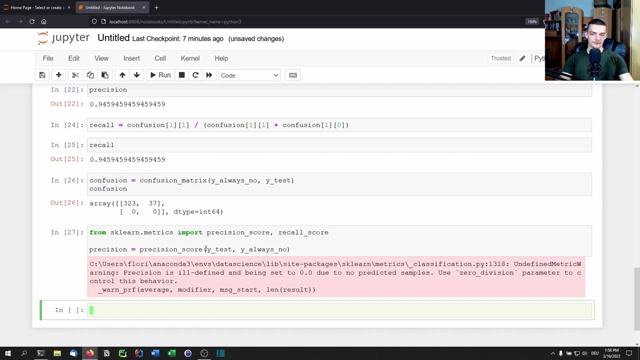 equals And the function is: let me just see where I had it. The function is precision score, And first we enter the y test, So the correct values, and second we enter the always no values, And in this case it doesn't work. Why? Because the precision cannot work if we don't. 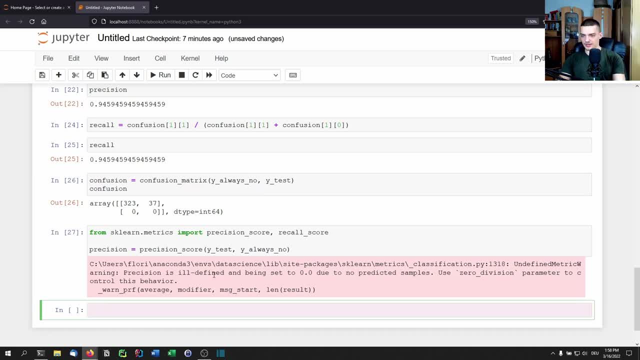 have a single classification, So in this case it doesn't work. However, if I now say recall, this is the correct value And in this case it doesn't work. So in this case it doesn't work. It is going to work. Recall: score y, test y: always no And the recall is zero. 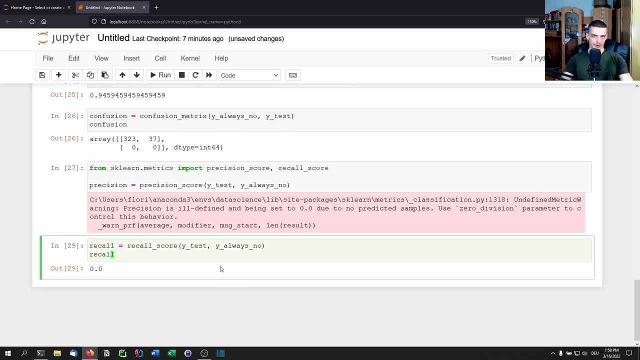 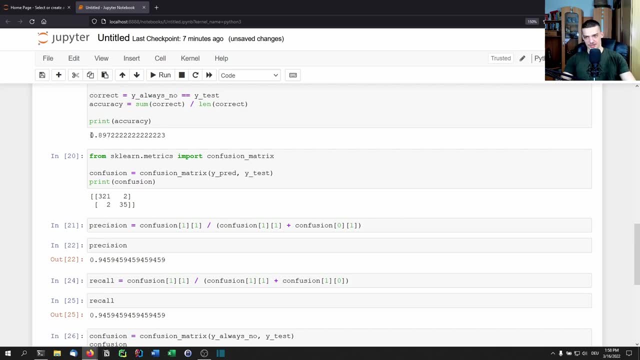 0% of the time when we see an eight, we actually recognize it. So this is pretty bad. If we look at the accuracy, we don't get that picture. 89.7% is not too bad. It's not perfect, It's not very. 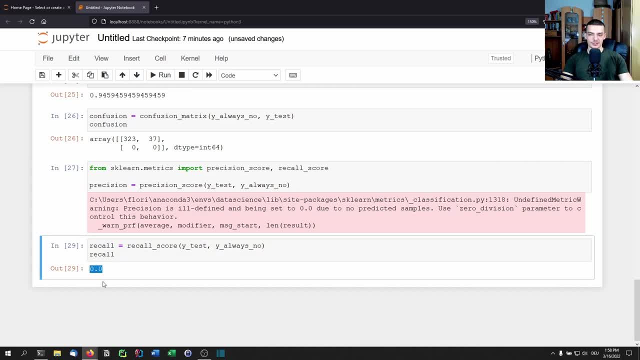 good, but it's not bad. But when we look at a recall of zero, this is horrible. This is a very, very bad model. Now we can also try the opposite. we can try to say always yes, So essentially y, always yes, is going to be once times the length of. 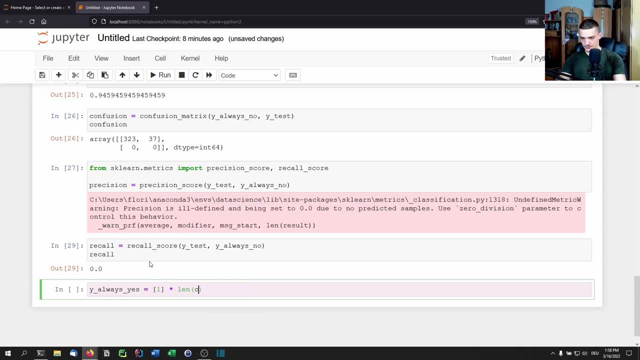 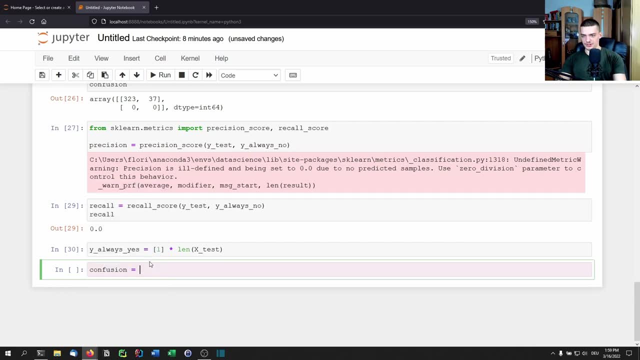 not this x test. there you go, And then we're going to get a different confusion matrix. So if I now say confusion equals confusion, matrix of y- always yes- and y test, then we're going to see that the first row is empty. So we always say it. 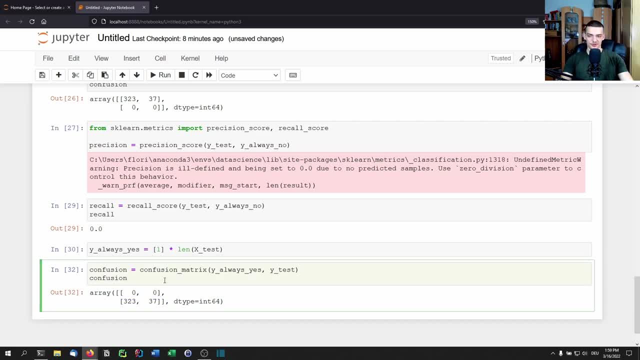 is an eight. Because of that, guess what? the recall is going to be phenomenal, because we recognize every single eight. If I now say recall score of y always yes And y test, and y always yes, because that's because we say it is a number equal to 0. And then this is going to: 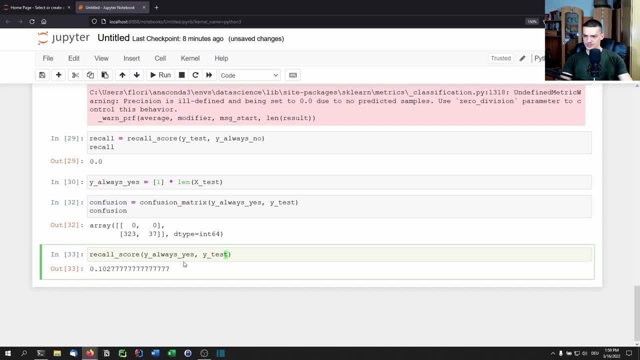 be an eight. So if I now say reasonable, then we're going to get a very bad one, This is not true. And then I'm going to say no, this is not true. Oh yeah, I messed up the order we need to do. 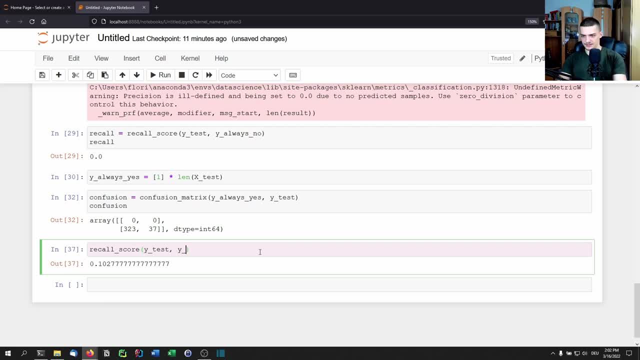 it the other way around. So first y test and then y, always yes. Then you can see we have a recall of 100%. Obviously, because whenever we see an eight we say it is an eight. so we never miss a single eight, But we do so for every number, which means that, in turn, if we now look at the precision score, 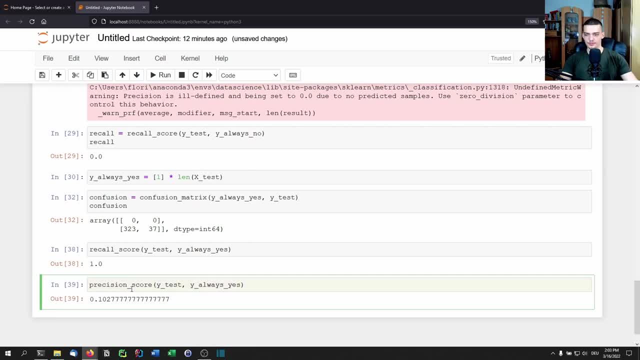 of y test and y always. yes, this is going to be a total of five, So we're going to get zero And yes, this is going to be horrible: 10, 10.27, because basically, whatever we see, we say, it's an eight. 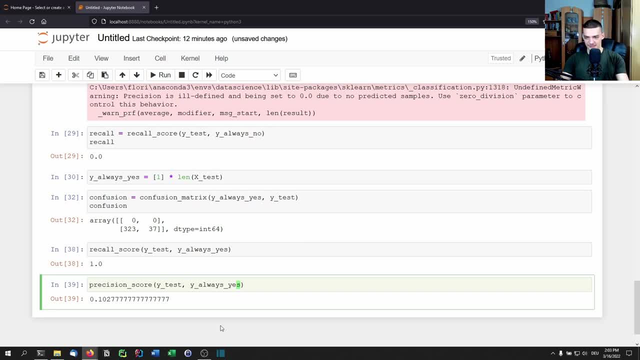 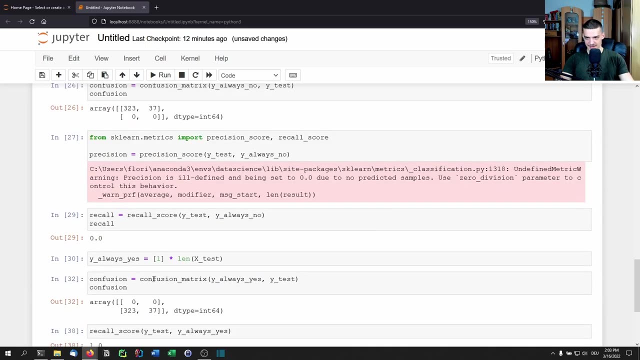 and obviously it is not because we have a lot of other digits and because of that the precision is very low and the recall is very high and the accuracy is going to be pretty bad here in this case, even though it's not the case for always, no, but the accuracy is going to be quite bad. 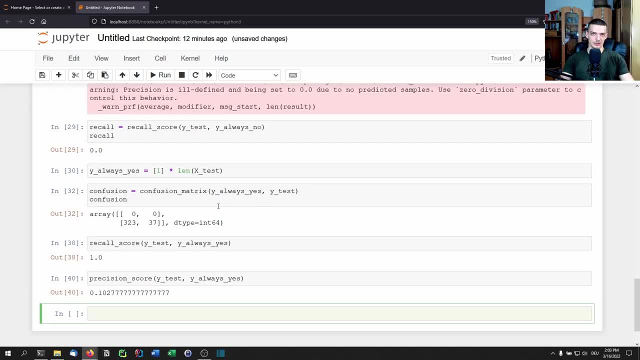 for this, because we basically do a lot of misclassifications in this case. so one last thing that we want to introduce here, which makes sense to introduce here, is the so-called f1 score, and the f1 score is the harmonic mean of precision and recall, and harmonic mean basically means that 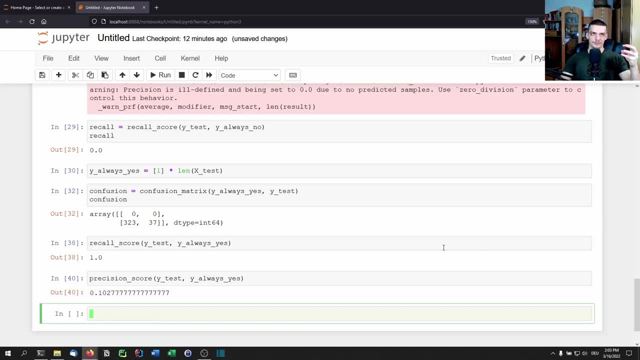 smaller values are, more are affecting the final result more, which in turn means that in order to have a high f1 value, we need to have a high recall and a high precision. we cannot achieve a high f1 score if one of the two values is very low, so we have to have both quite high in order to reach a high f1 value. 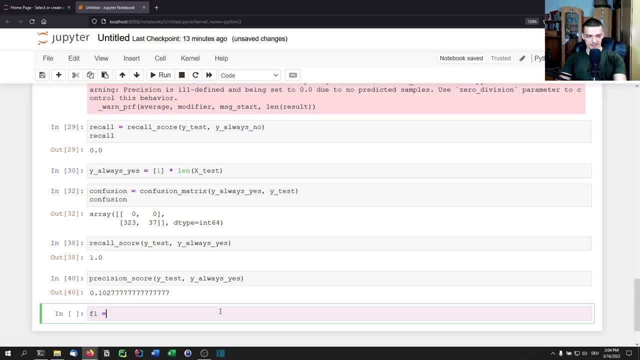 and the formula is essentially just: f1 equals two divided by, and then one divided by precision plus one divided by recall, like that. and for that we're going to say, oh sorry, now i've messed this up again, come on, why always? yes, there you go. recall is that. 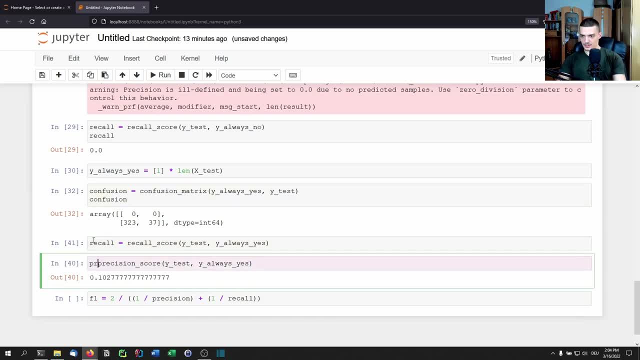 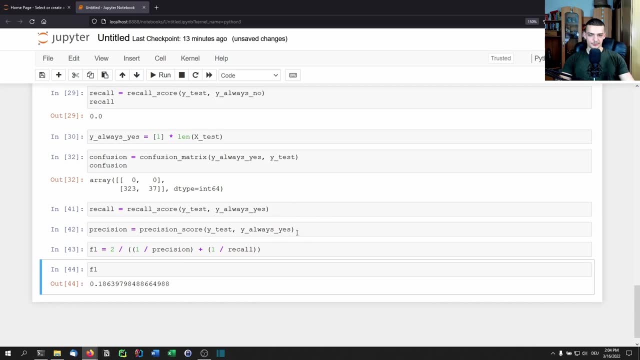 and precision is that and the f1 score is going to be that. and in this case the f1 score is very low because the precision is very low. if we have a high precision and a low recall, it's also going to be very low. if we have a high precision and a low recall, it's also going to be. 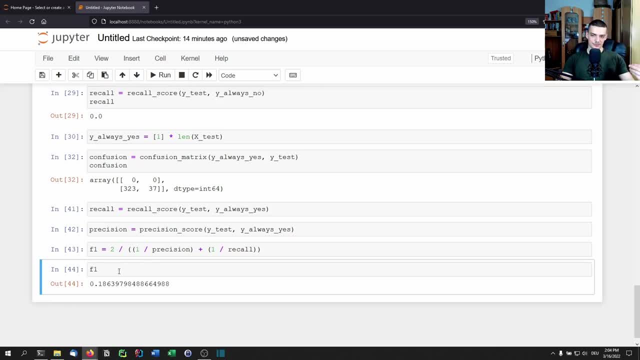 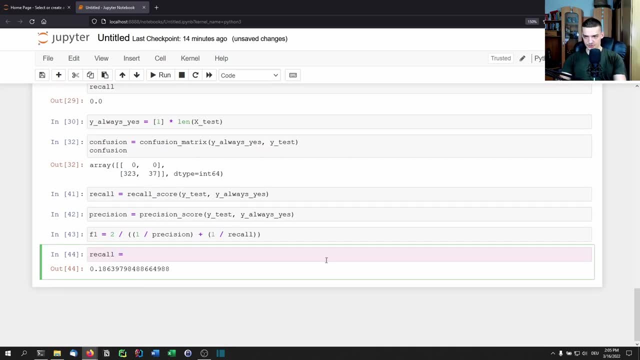 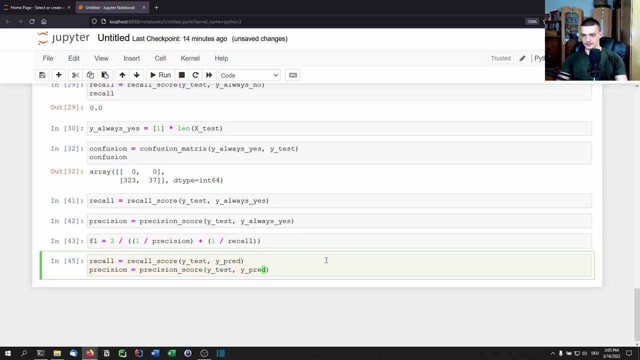 going to be very low. If both are decent, we're going to have a decent F one score. So actually we can do the same thing now for 40 for the actual values of the key neighbors classifier. So recall score for y test compared to y predictions in precision. Same thing like that. And then 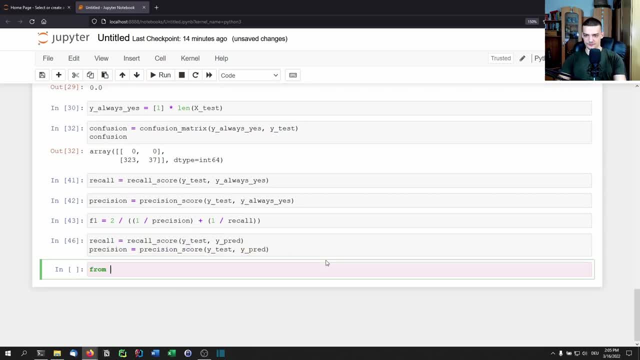 what we can also do here. we can import the F one score from sklearn. So from sklearn dot metrics, import F one score, And now we can just say: print F one score. Oh, oh, actually we don't need that. I forgot that. we don't need that. We can do it directly like this: 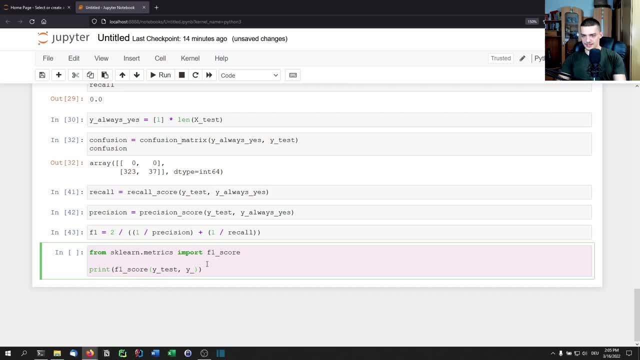 it's going to do everything behind the scenes, So why test? but I think it can actually be useful. can I somehow get this back? No, okay, But when we now go and say why tests and why predictions we get a high F one score because the precision and the recall are pretty high. we can see them. 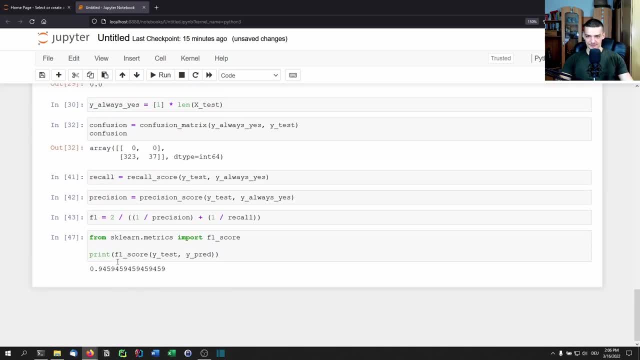 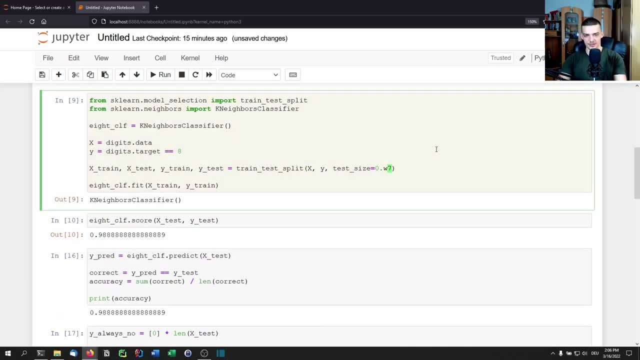 here. Both are high In this case, both are the same And because of that we get the same F one score as well. But we can change things up a little bit. we can make it harder by increasing the test size, meaning that we're going to train, in this case now on 30% of the data to predict 70%. 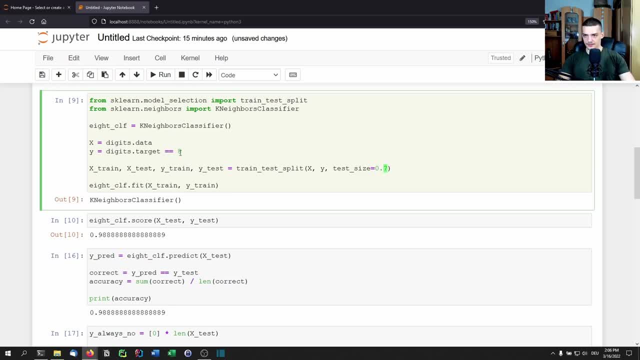 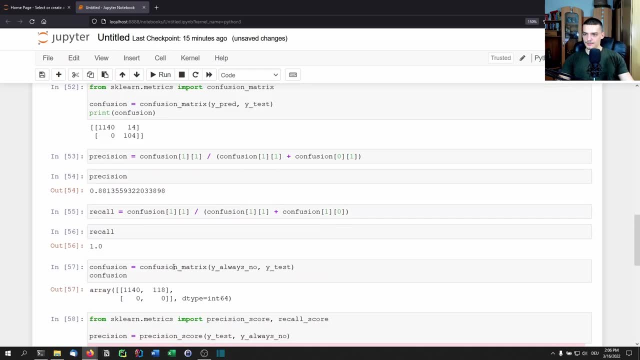 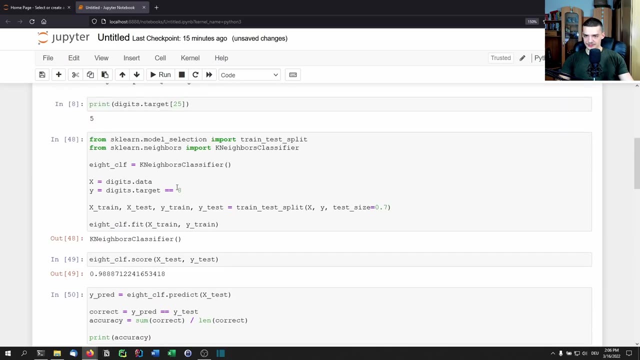 of the data, which is way harder. And if we do it like that, let's run all this here. we get a lower score, But we should probably get different precision and recall. There you go: Oh no, it's the same, Let's go with a different digit. Maybe let's go with a five. 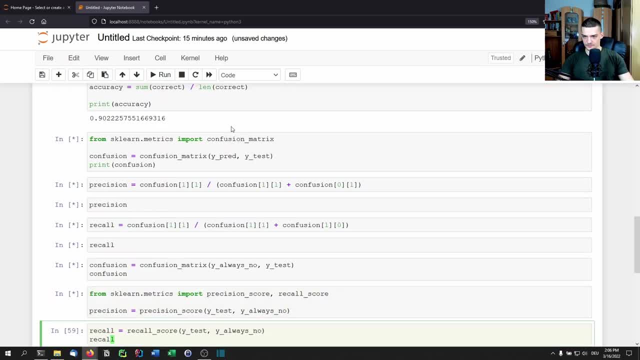 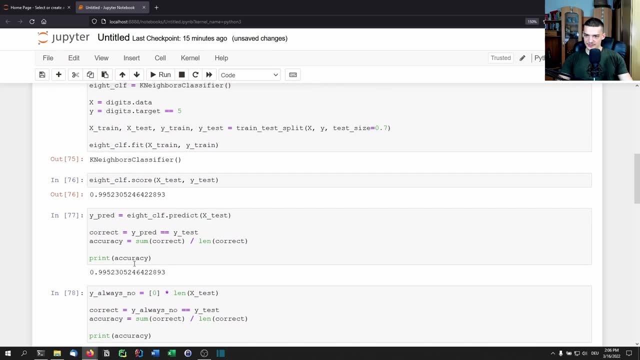 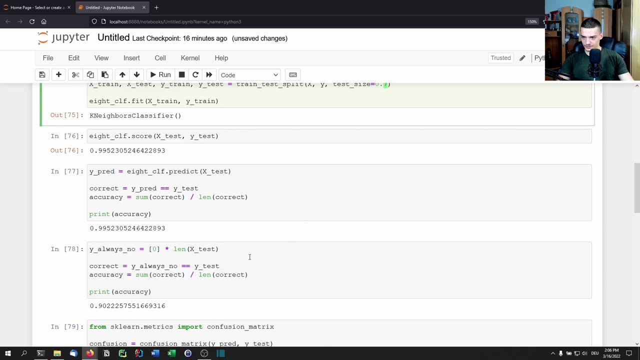 So let's just run this from the beginning again, Let's just force different results. Okay, here we have a pretty high F, one score, And we have again the same same recall and the same precision. So let me just see real quick here. No, I'm looking at the wrong values. What am I doing, mate?